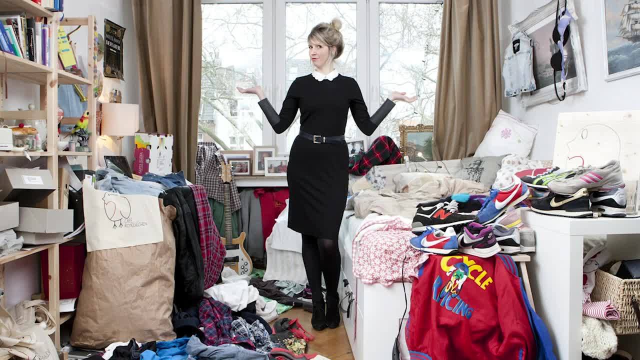 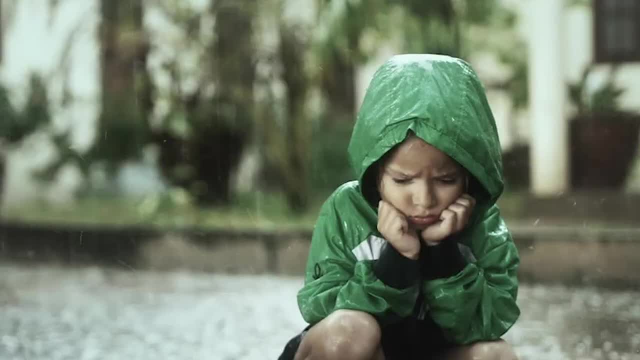 Everything is a mess. Where did I put that thing? Why can't I find that other thing? Oh no, I forgot about that assignment. Why didn't I remember that I don't have the time to get everything done? I've got to do something about this. Is this you? It's definitely me sometimes. 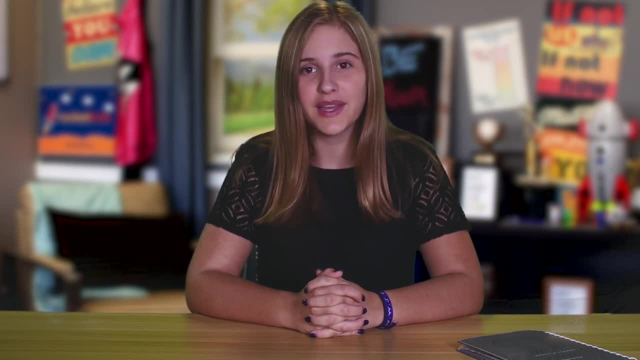 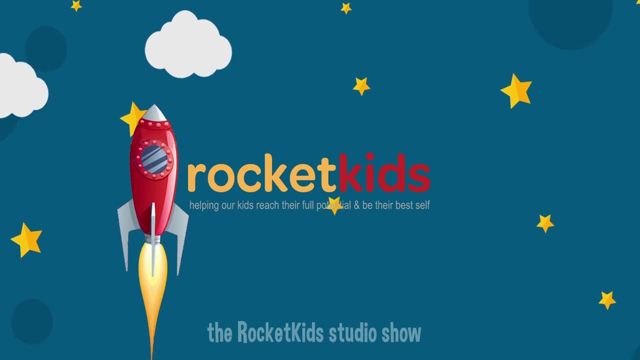 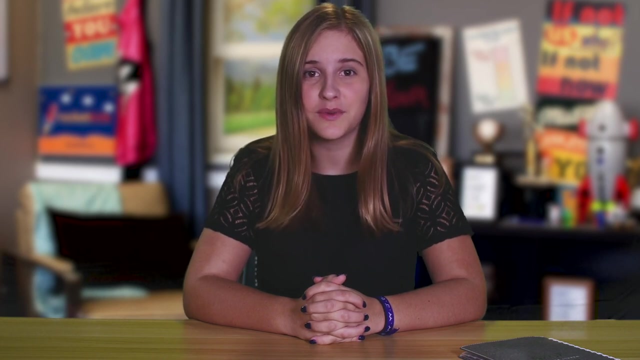 The good news is we're in luck because I have four ways we can all get organized. I'm Morgan, this is Rocket Kids and let's get this started. So how do we get organized? For starters, we can do these four things to get some order. 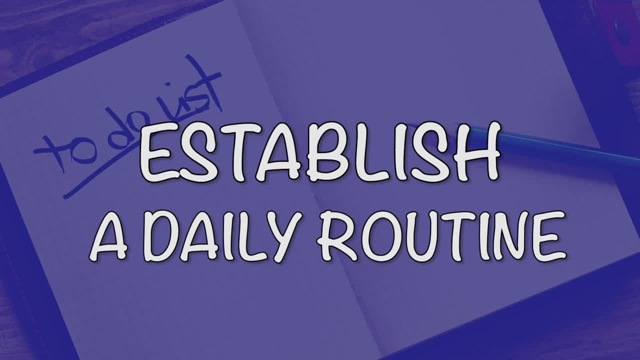 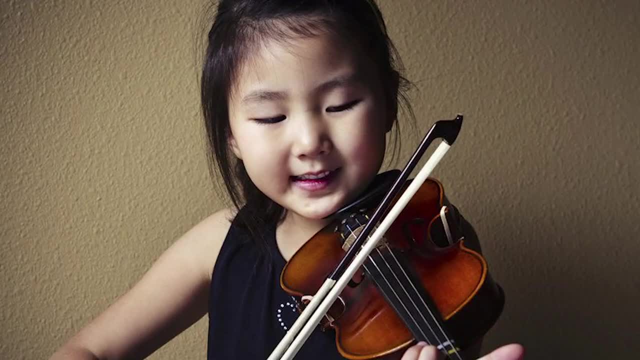 to our disorder Number one: establish a daily routine From our rise and shine time until lights out time. take notice of when you get dressed, eat breakfast, practice something you love, do your homework and have time to play with your friends When we know what we have to do. 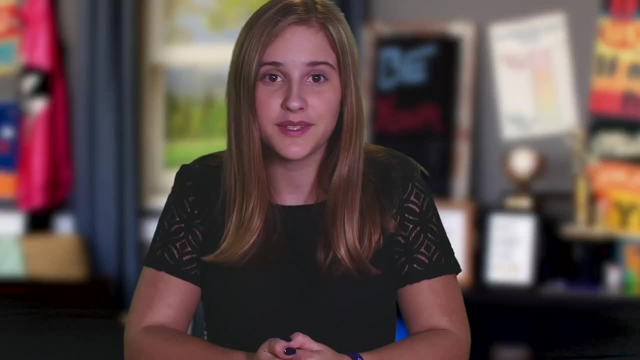 and when we do it we can make a regular schedule. This helps us know what to expect throughout the day, so we don't have as many of those we didn't see that coming kind of things. So how do we get organized? For starters, we can do these four things to get some. order to our disorder Number one: establish a daily routine From our rise and shine time until lights out time. take notice of when you get dressed, eat breakfast, practice something you love, and when we do it, we can make a regular schedule. This helps us know what to expect throughout. 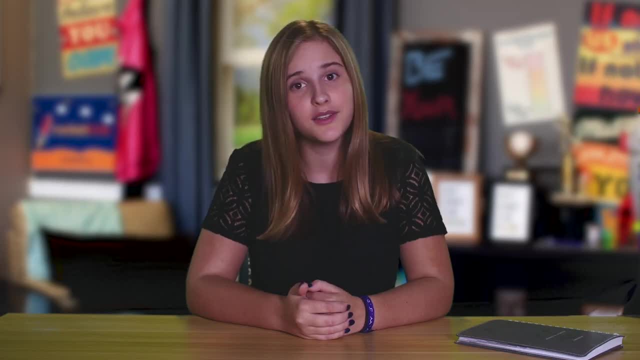 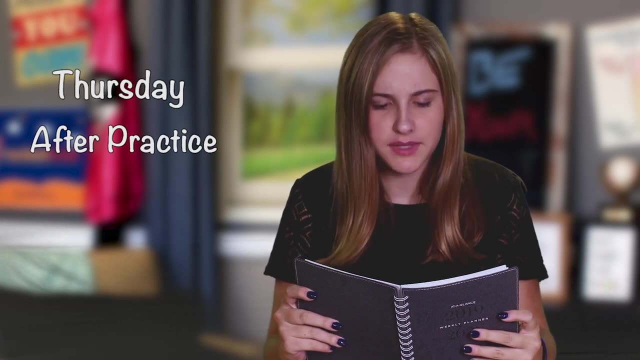 the day so we don't have as many of those. we didn't see that coming kind of things. And when you're asked to attend a meeting to solve world peace, you can look at your calendar. This is my calendar, Let's see. I can do Thursday after soccer practice, but I need to do that meeting. 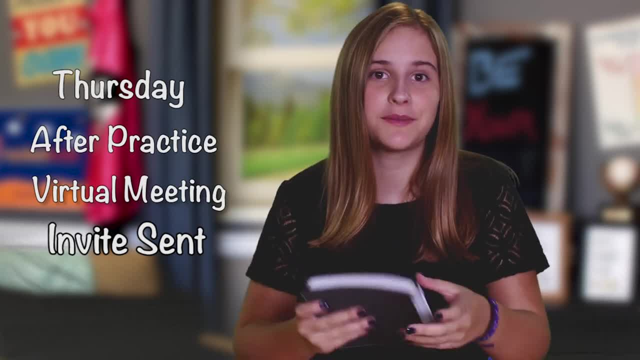 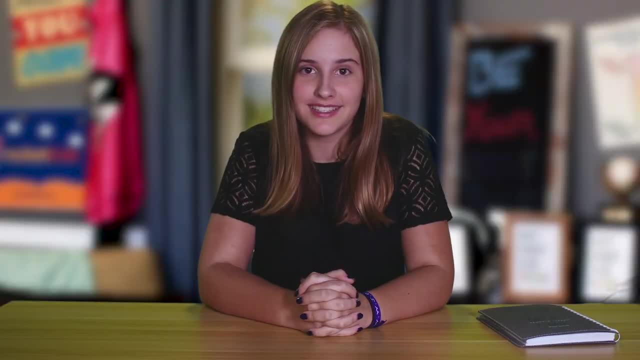 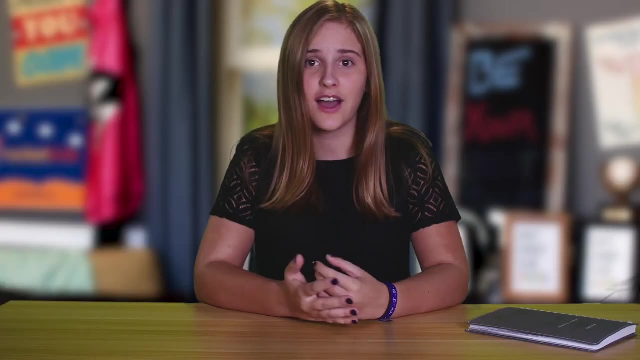 virtual Okay invite sent, So looks like next Thursday after practice I will be solving world peace. Just know this: when we establish daily routines and stick to them, we never miss anything and catch everything. Number two: manage your time. Remember that. 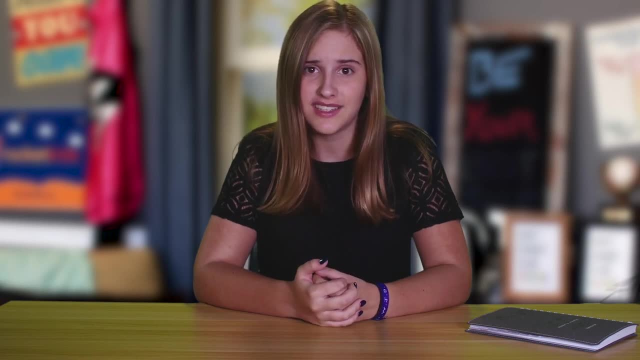 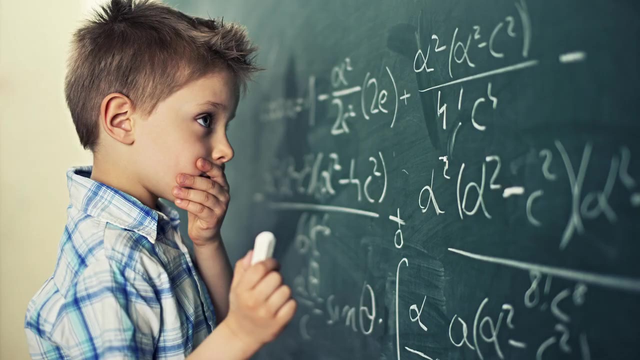 how am I going to get all this done? and I don't have the time. How about this? Write it down. Write down important tasks and then estimate the time it will take to do each one, Monitor how close you are on those estimates and then make any adjustments for the next time Missing those. 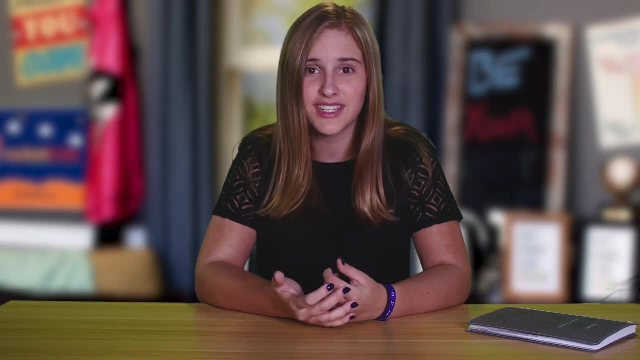 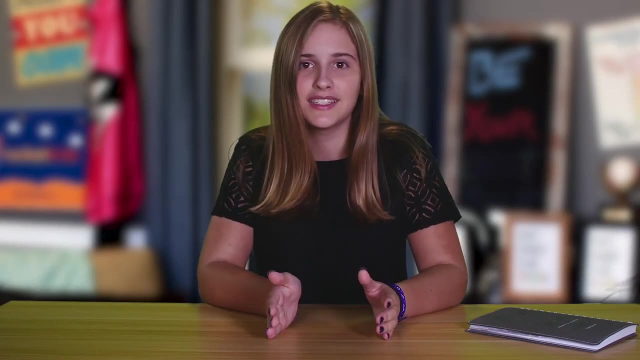 assignments or cramming to study for that test, always rushing to get that project done. break your time into steps with your own personal due dates, Kind of like a beginning, middle and end, where the end is crushing that project And you did it without being overwhelmed and